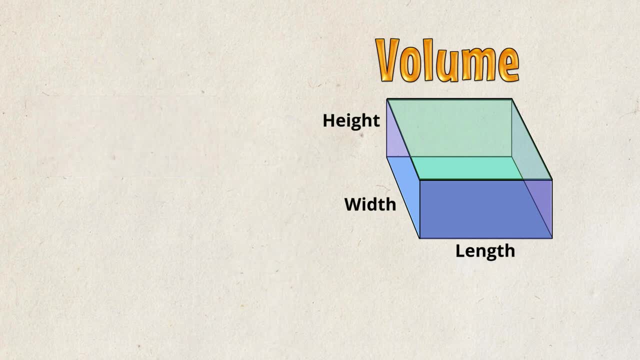 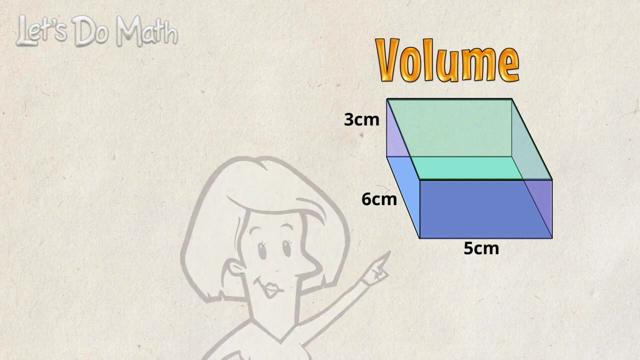 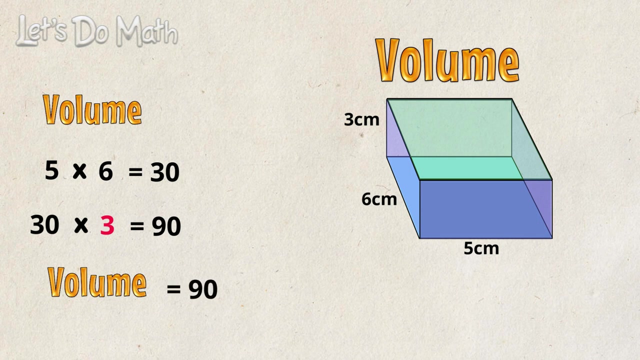 we have 3 dimensions. to multiply 3cm and a height of 3cm To find the volume. Let's start with the rectangle base. Now we multiply that by the height measurement. So we say: Why is it cubed? If we were to fill up, 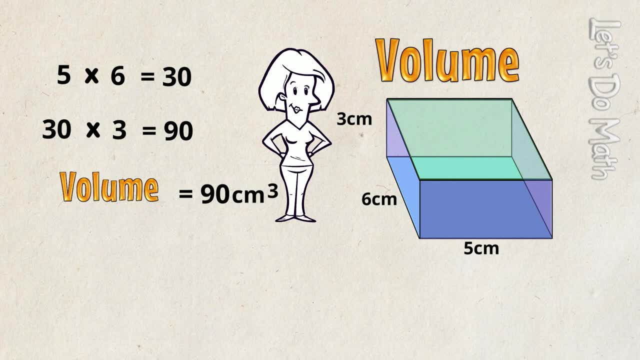 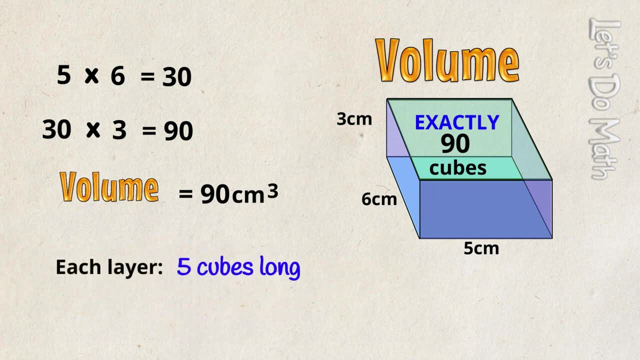 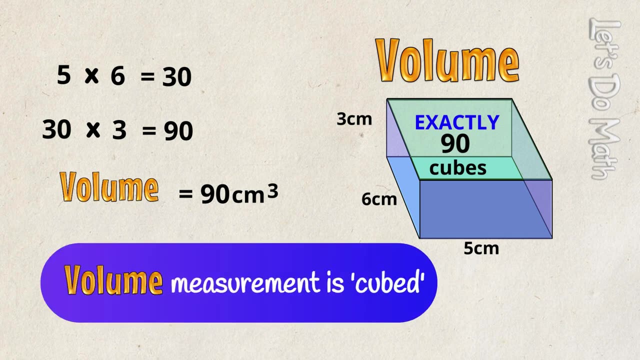 this box or rectangular prism with 1cm cubes. it would take exactly 90 cubes. Each layer would be 5 long and 6 wide and there would be 3 layers. That's why the volume measurement is CUBED. We show this in writing with a little superscript. 3. 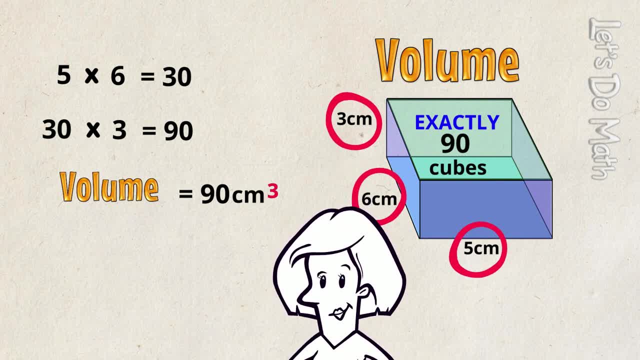 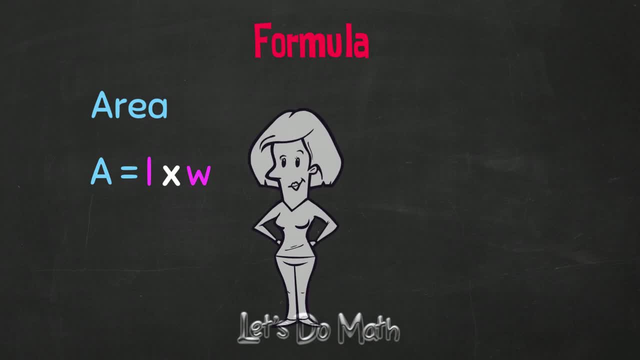 which makes sense because we're multiplying 3 dimensions to find the volume. You know the formula for AREA- LENGTH x WIDTH- and there's a formula for VOLUME too. VOLUME is LENGTH x WIDTH x HEIGHT. You may also see the version that's quicker to write down. 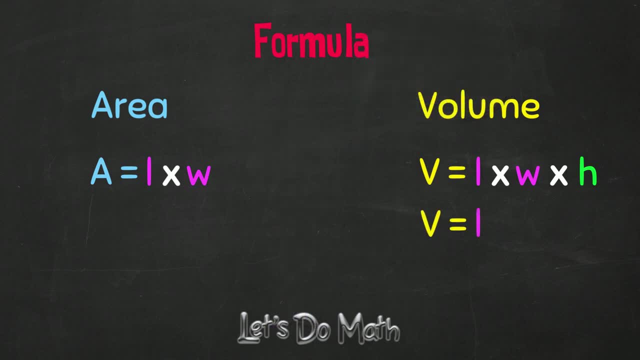 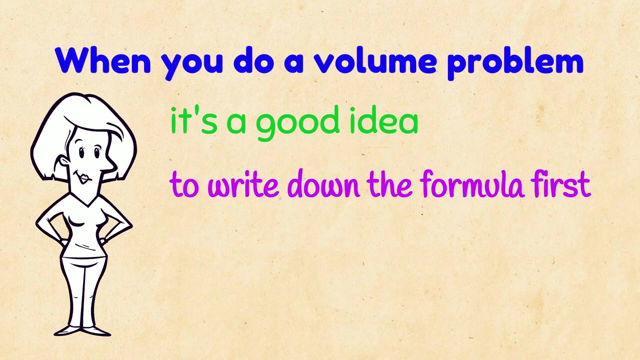 V equals LWH. They mean exactly the same thing. Multiply LENGTH, WIDTH and HEIGHT to get the volume. When you do a volume problem, it's a good idea to use a formula to get the volume. It's a good idea to write down the formula first. It helps make sure you do everything you need to do. 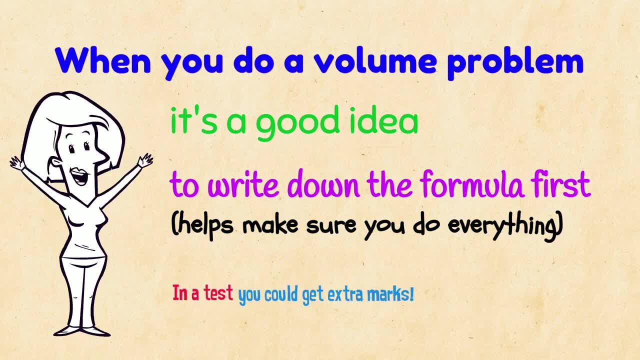 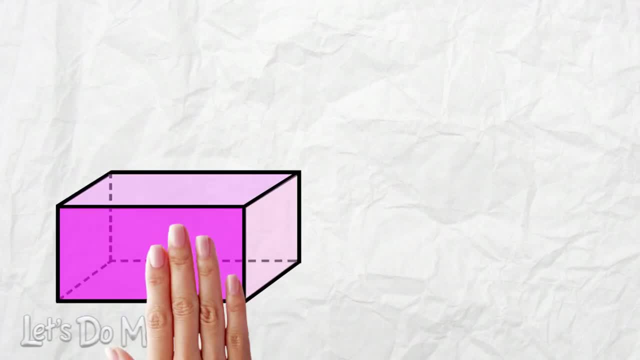 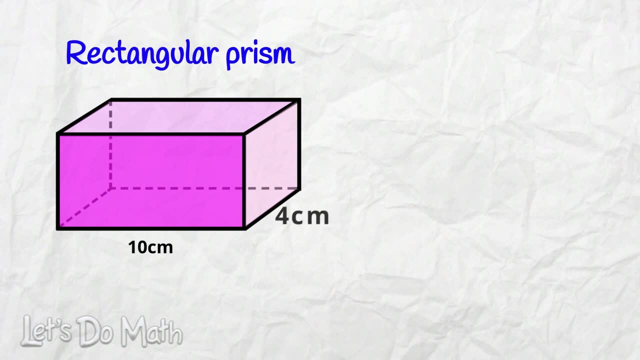 and in a test or exam you could get extra marks for including the formula Ok. one last example, then it's over to you. This box, or rectangular prism, has a length of 10cm, a width of 4cm and a height of 5cm. 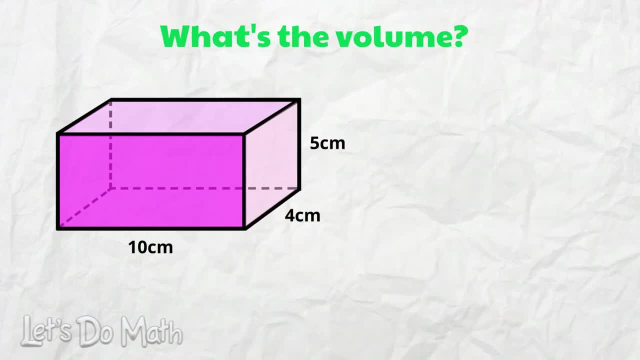 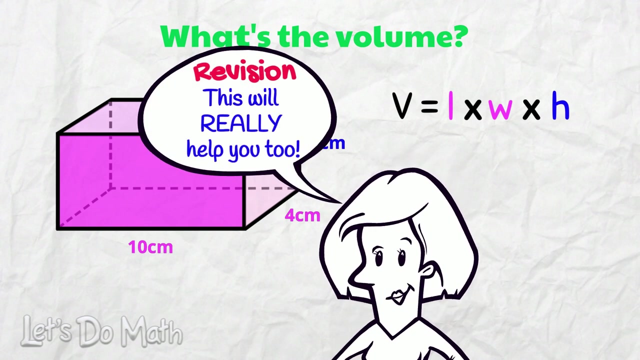 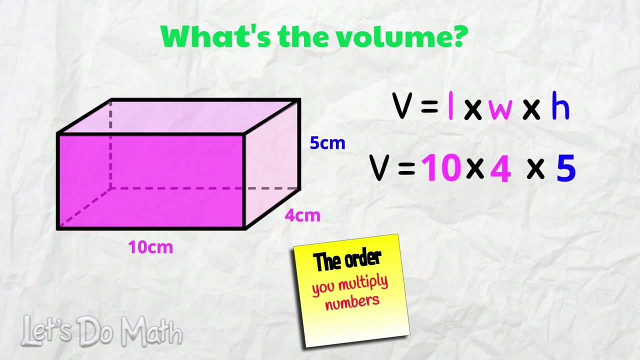 What's the volume? First, the volume is the formula Underneath each dimension. I'm going to write the values from the diagram. This shows my thinking clearly and your teacher will love this, And when it comes to revision, this will really help you too. The order in which you multiply numbers.